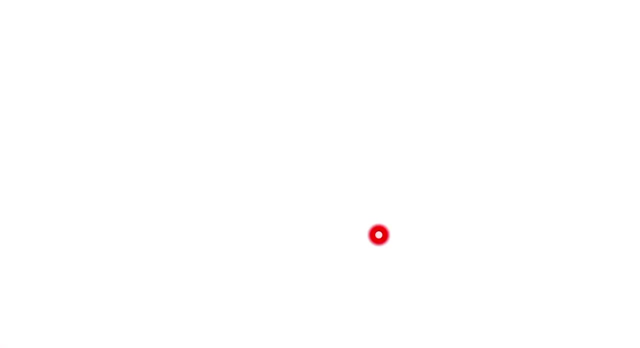 Welcome back. Today we are going to solve this question. In this question we have to find the value of x. Can you solve this? If you can, then pause the video and take a try, Otherwise let's see the solution. So this is our question: x to the power, x to the power, 5 is equal to 100. 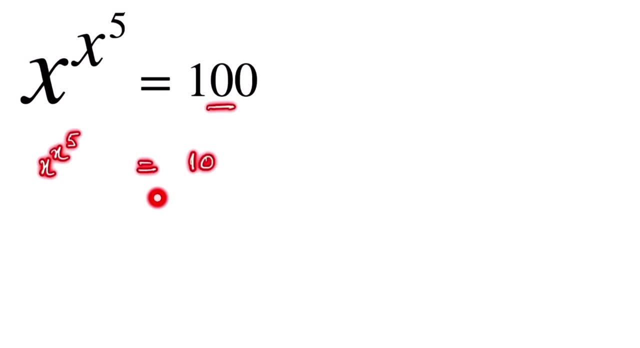 So here, x to the power, x to the power, 5 is equal to 100, can be written as 10 to the power 2.. So here now we power with 5 on both side. Just look like this. So here now we exchange the. 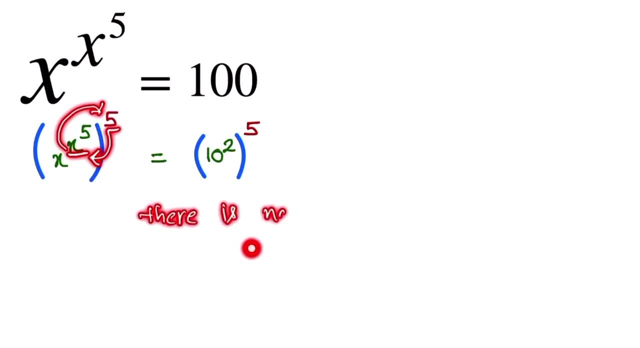 position of power. So when we exchange the position of power there is no effect in equation or system. So here, x to the power 5, the whole power is x to the power 5 is equal to now. we multiply this power 10 to the power 10.. So here we notice in this equation: 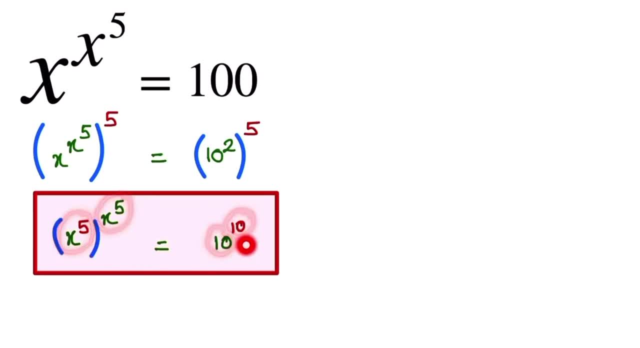 x to the power 5 and this one is x to the power 5. and here is 10 and 10.. So now we can say that, yeah, we had founded the value that x to the power 5 is equal to 10.. So here is x to the power 5,. 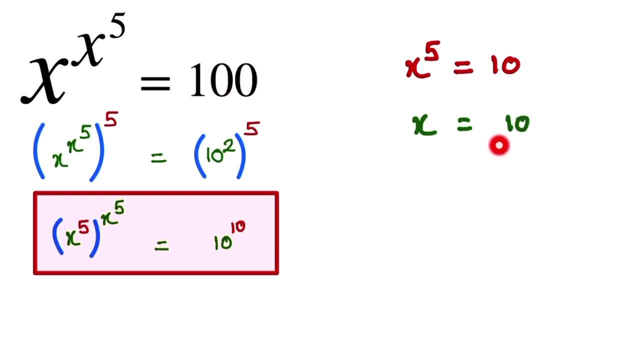 here is 10, x to the power 5 and 10.. So here x is equal to 5 under root 10, 5th under root 10.. And this one is our final value of x. So now we check this. So here is x is. 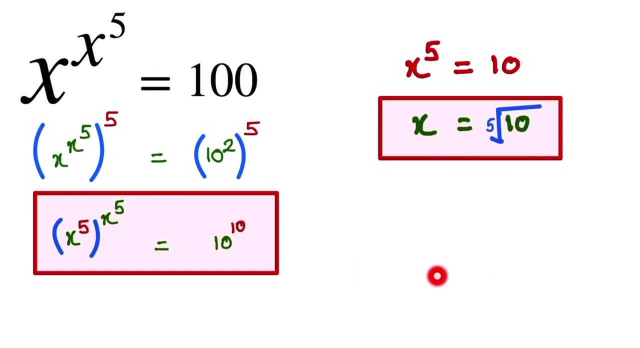 equal to. we put the value on the x. so here 5 under root 10, the power 5 under root 10, the whole power is 5 and here is equal to 100. so here 5 under root 10, and here this 10 and 1 by 5 into 5 and 5. 5 is cancelled. 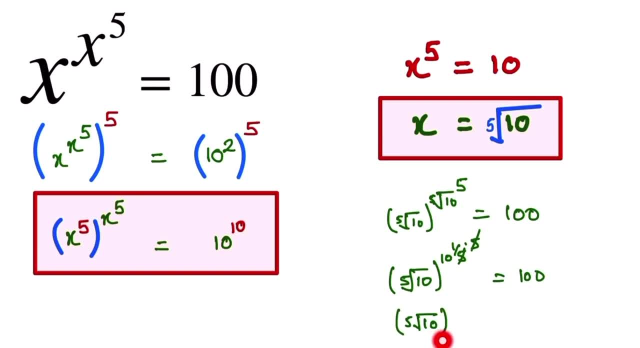 so here is 5 under root 10, and here the power is 10 is equal to 100. so now 10, the power 1 by 5 into 10. so here is 10 is cancelled out by 5, 2, so 10 square is equal to 100. so 10 square is equal. 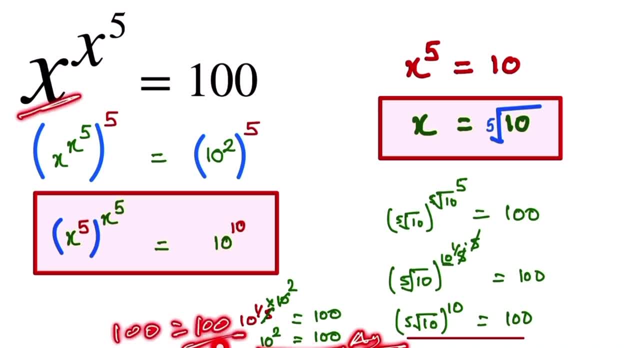 to 100, 100 is equal to 100. so here we prove. the final answer of x is equal to 5 under root 10, and this one is final answer. thank you so much for watching my video. if you like the video, then subscribe our channel and hit the bell icon so that you don't miss any of my new videos.